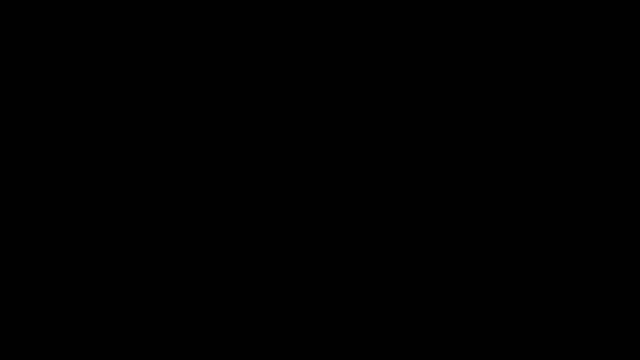 In this lesson, we're going to focus on differentiating inverse trigonometric functions, So let's get right into it. What is the derivative of arc sine of x, cubed? Go ahead and try this problem. Now you need to know the formula. If you know the formula, life is easy. 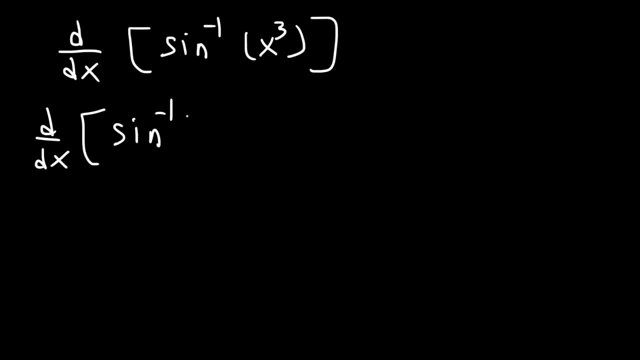 The derivative of some generic arc sine function. let's say arc sine u. it's equal to u prime divided by the square root of 1 minus u squared. So all you need to do is identify u and u prime. Well, the first part is straightforward, because u is the stuff inside of the arc sine function. 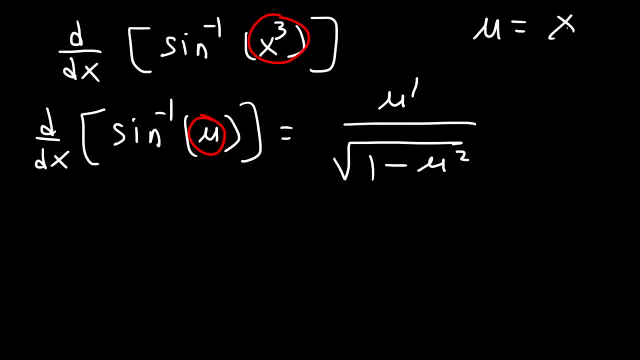 So we can see that u is equal to x cubed. Now u prime the derivative of u. that's going to be the derivative of x cubed, which is 3x squared. So now we can get the answer. 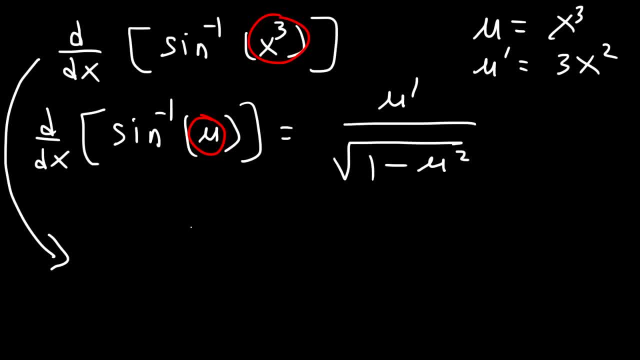 So the derivative of arc sine x cubed is going to be u prime, which is 3x squared divided by the square root of 1 minus u squared, or 1 minus x cubed squared. So the final answer is 3x squared divided by the square root of 1 minus x. to the 6th power. 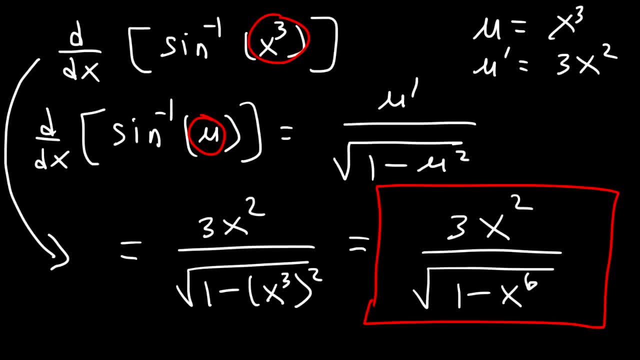 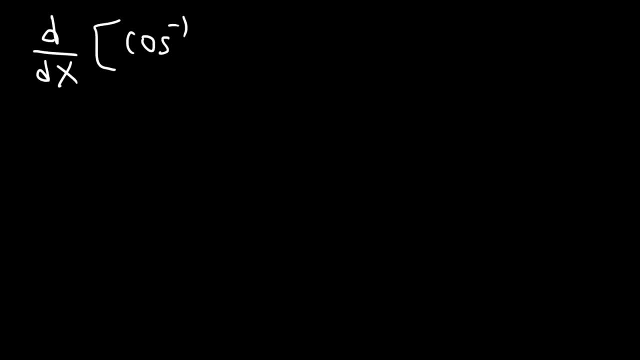 And so this is the answer. Now let's try another example. What is the derivative of arc cosine 5x minus 9.. Go ahead and try that. So here's the formula that you need. The derivative of arc cosine of u is very similar to the arc sine of u formula. 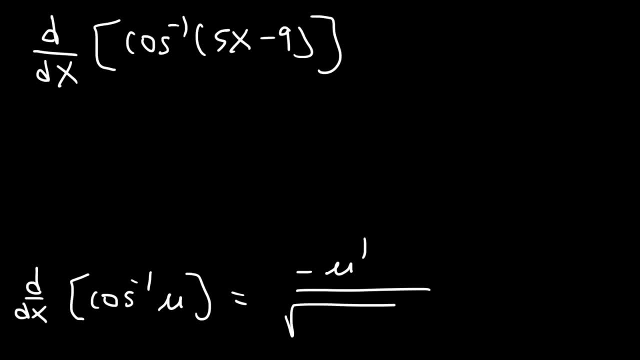 It's going to be negative u prime instead of positive u prime divided by the square root of 1 minus u squared. So in this example, u is 5x minus 9.. That's the stuff inside. That's the stuff inside of the arc cosine function. 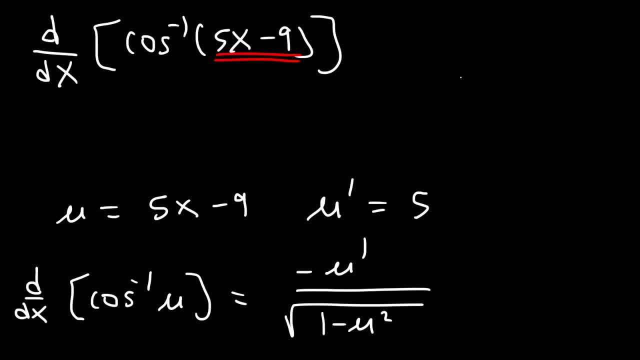 And the derivative of 5x minus 9 is simply 5.. So the answer is going to be negative: 5 divided by the square root of 1 minus 5x minus 9 squared, And that's the solution for this problem. 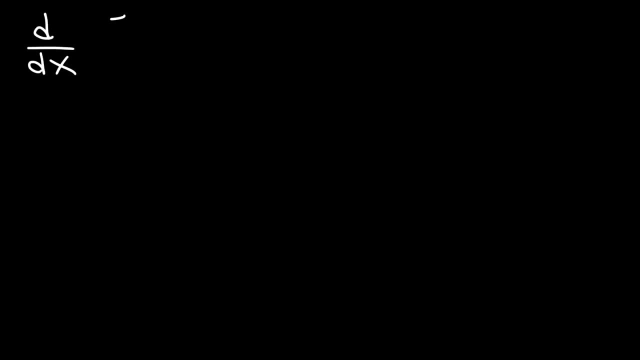 Here's another problem that you can work with. What is the derivative of arc tangent square root x? So if you don't have the formula, check out your textbook. It should be in it. But here it is. for arc tangent, The derivative of arc tan or inverse tan of u is going to be u prime divided by 1 plus u squared. 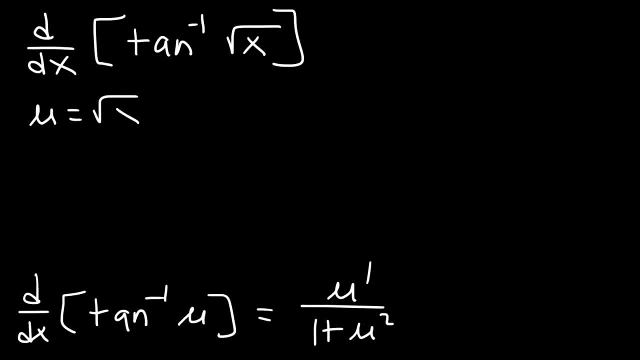 So we can see that u is the square root of x, which, if we rewrite it, that's x to the 1 half. Now u prime, that's I brought u to the half for some reason. u prime is the derivative of x to the 1 half. 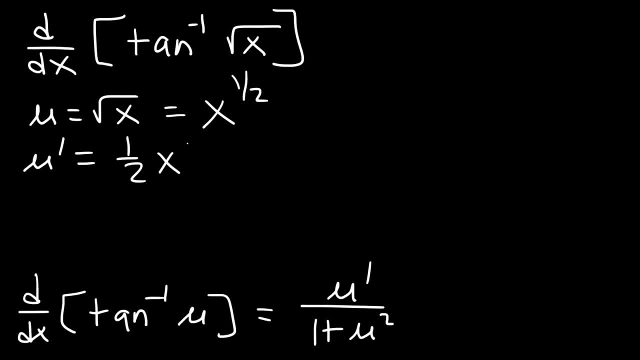 So, using the power rule, it's going to be 1 half, x to the minus 1 half, And we can rewrite that as 1 over 2, x to the positive 1 half, And then, converting it back to radical form, it's 1 over 2 square root x. 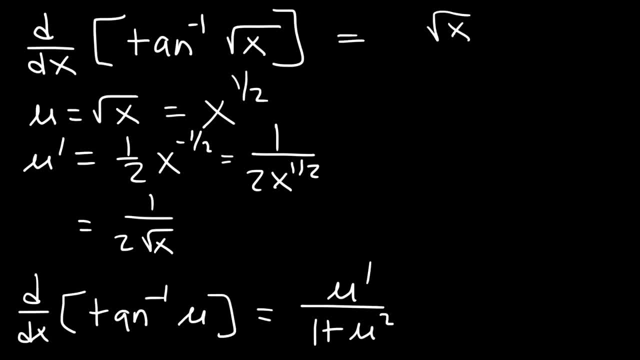 So now let's use the formula: It's u prime, which is square root x, divided by 1 plus. well, actually I take that back: u prime is this thing right here. So that's 1 over 2 square root x, and then divided by 1 plus u squared. 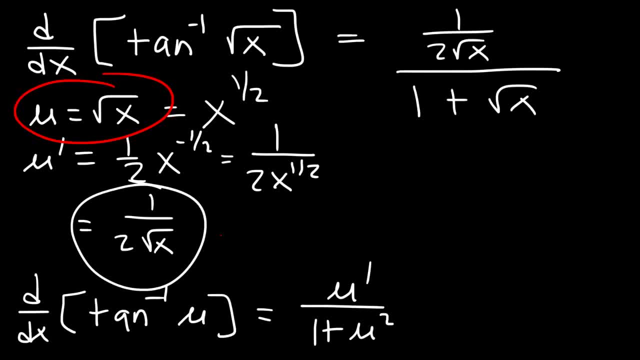 So u is the square root of x, And once we square it, it simply becomes x. So this is 1 over 2, square root, x divided by 1 plus x. Now we could simplify the expression. Now let's multiply the top. 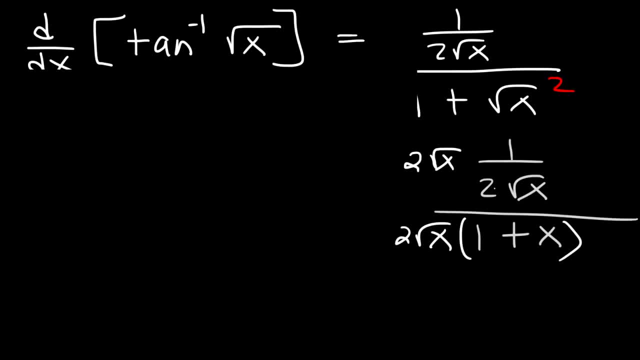 And the bottom by 2 square root x, So we can get rid of the fraction in the numerator. So this is going to be 1 over 1 plus x times 2 square root x. And if you need to rationalize the expression, you can multiply the top and the bottom by the square root of x. 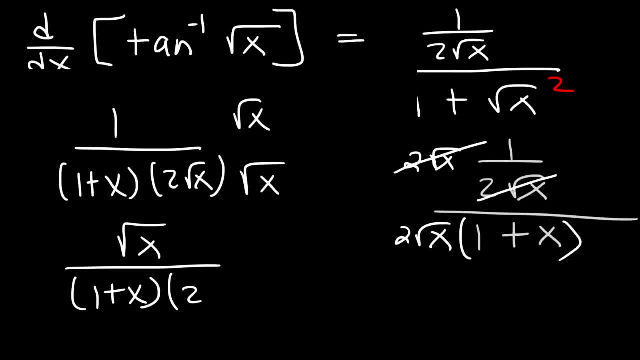